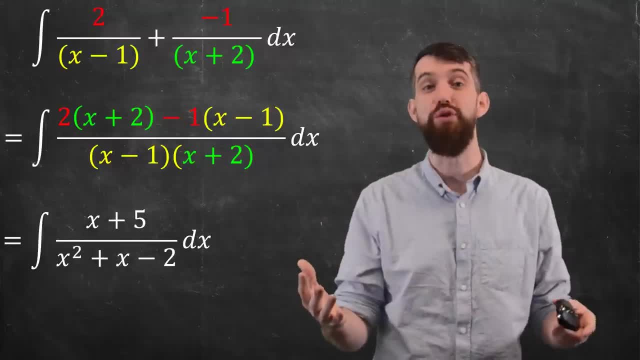 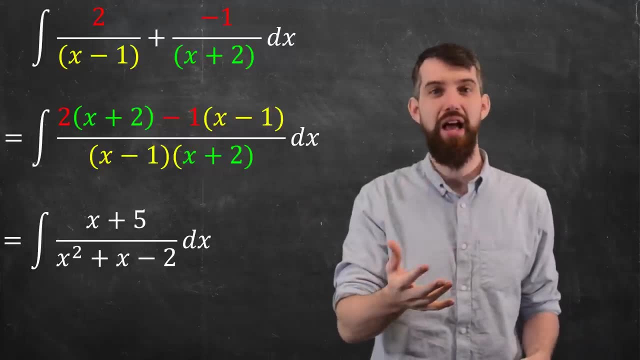 du doesn't match the numerator. Maybe I could think of a way to do it, but it would be a bit challenging. However, the top one is something I can do. For example, if I focus on the left-hand side, if I set u equal to x minus 1, then this is just going to be twice the logarithm. 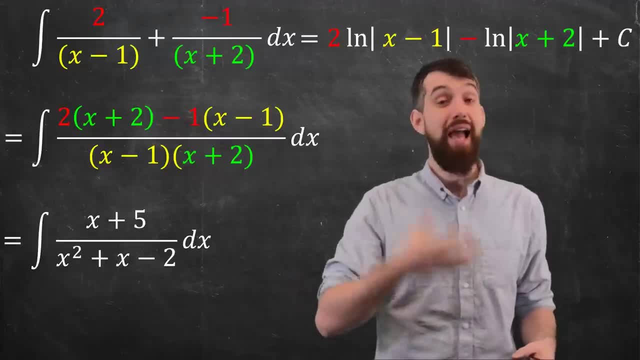 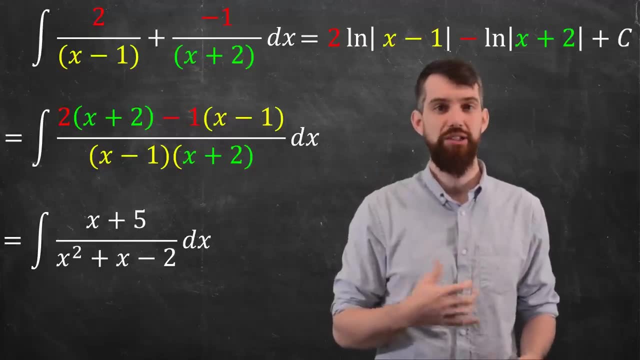 of the absolute value of x minus 1. after a little u substitution For x plus 2 is my u, then I'm going to get minus logarithm of x plus 2.. And then finally plus c. So the whole point is that this bottom one is hard to do. but 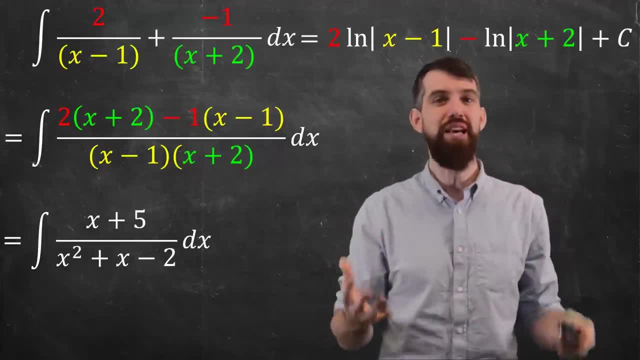 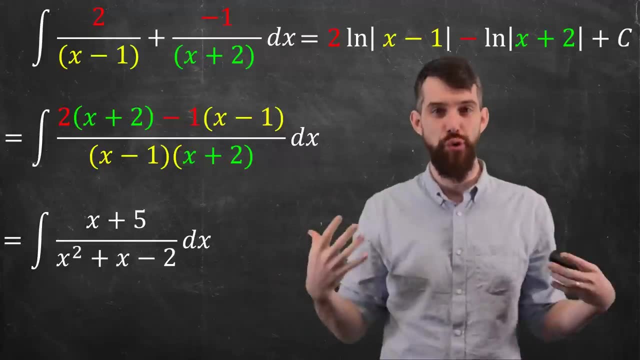 the top one is actually straightforward. So then, if I was given an integral that looked like the bottom here, one of these challenging ones, then what I want to do is try to do this process where I undo a lowest common denominator trick, and that's going to turn. 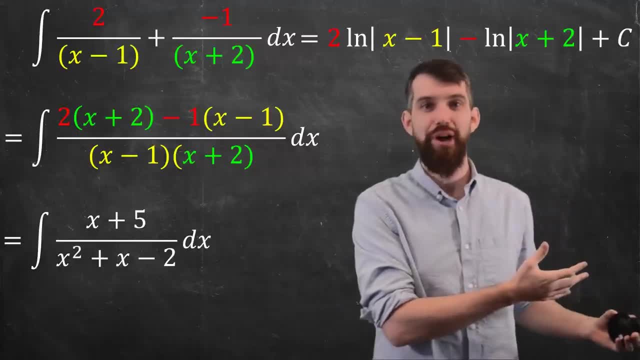 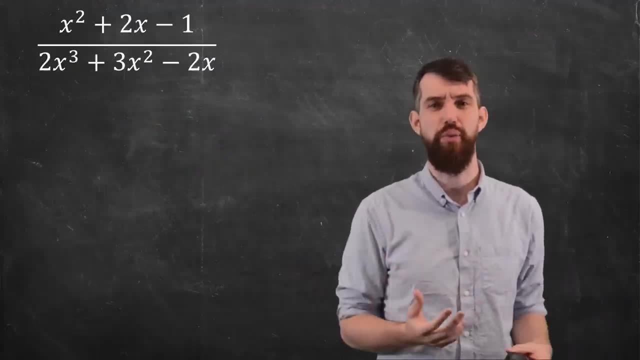 it into this top form that I do know how to do. So how, in general, do we undo finding lowest common denominators? Let's actually do it in a harder example. Let me illustrate the point In this particular example. I've got some quadratic on the top. 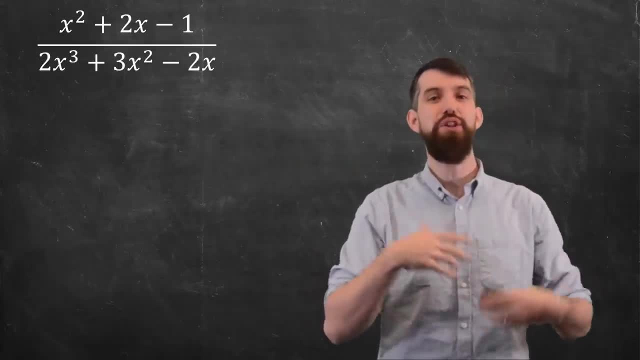 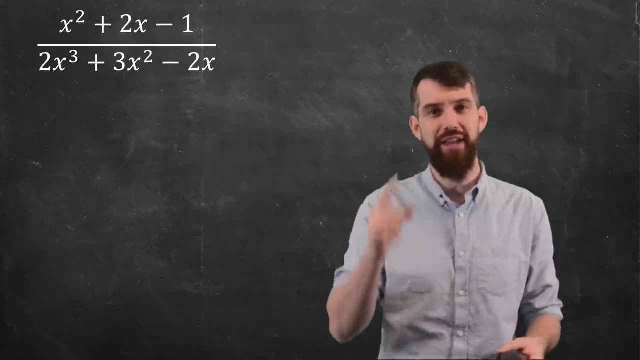 and a cubic on the bottom. Now, because I'm undoing lowest common denominators. I actually don't really care what the numerator is. Maybe I could try to factor it. It looks like it would be a bit messy in this case, but whatever, It's the denominator I want to factor. I notice. 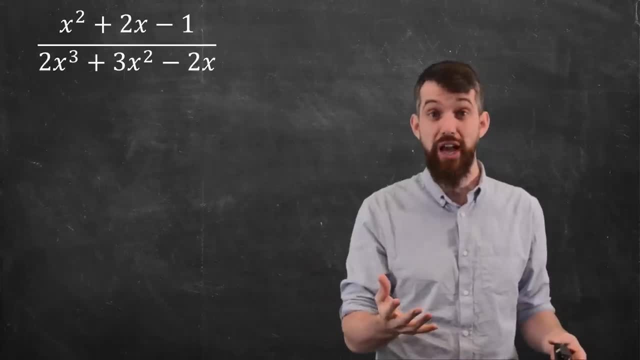 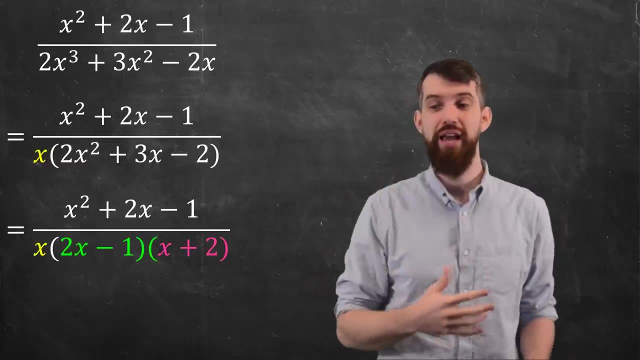 that it's a cubic and that there's an x in every term. So the first thing I'm going to do is I'm going to factor out an x and then that quadratic in the denominator. I can factor that out And it's going to give me a 2x minus 1 and an x plus 2, and then multiply by the x. Now, 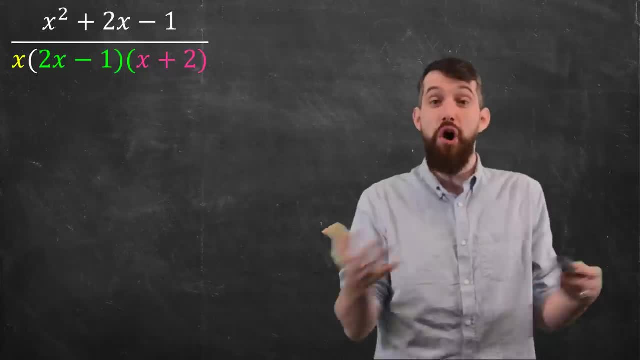 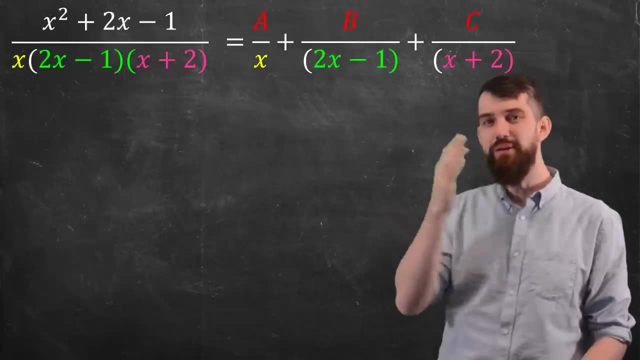 this is what I want to focus on. I want to undo a lowest common denominator like this, That is to say, I want to find three other numbers. I want to find this- a, b and c- and I want to write it in this right-hand way, such that the thing I began with is the. 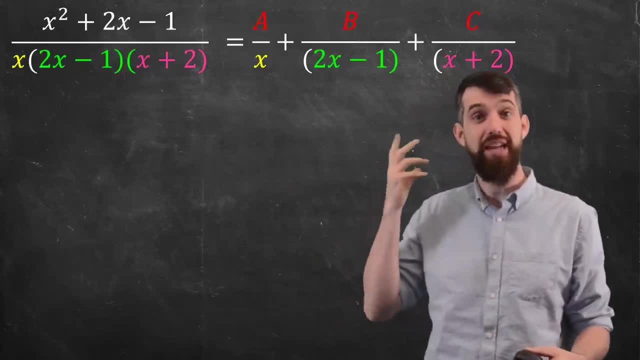 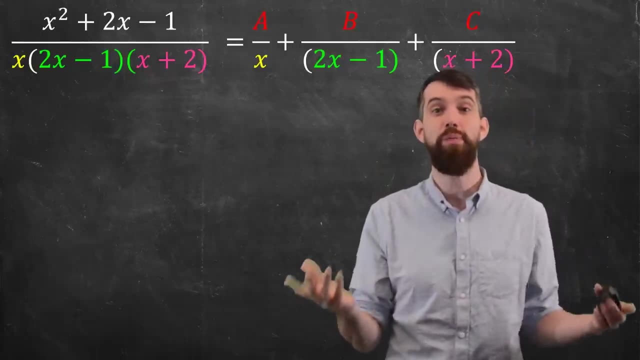 result of taking the lowest common denominator to the right-hand side. How can I do this? Well, if I was taking the lowest common denominator, what I would do is I would multiply both sides by the denominator On the left-hand side, taking the denominator. 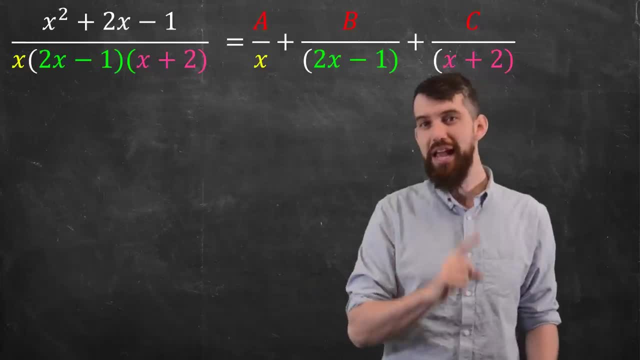 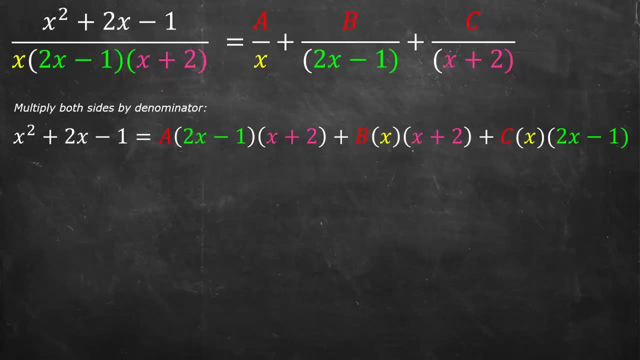 and multiplying it just gets rid of it. But on the right-hand side it's a little bit more complicated. I'm going to step away for a moment here because there's going to be a lot of algebra on the screen, but the basic idea is that for the a over x term, when I 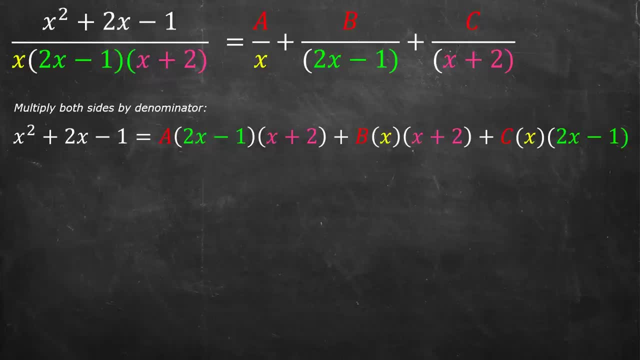 multiply by the denominator, the x cancels and I'm left with a multiplication of 2x minus 1.. For the b term, the 2x minus 1 goes away. when I multiply by the denominator, I'm left with an x and an x plus 2, and for the c term it's x and 2x minus 1.. 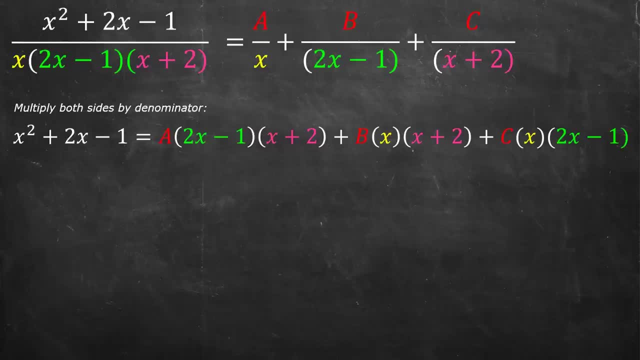 Now I'm going to clean it up a little bit. I've got an a times something, a b times something and a c times something and I'm going to expand all three of those. So the left-hand side remains the same, becomes a times a quadratic, b times a quadratic and c times a quadratic. 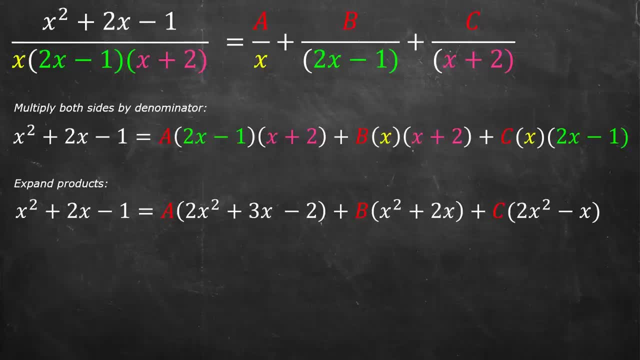 Now I've been focusing on the a, the b and the c. Now I've been focusing on the a, the b and the c. Now I've been focusing on the a, the b and the c. 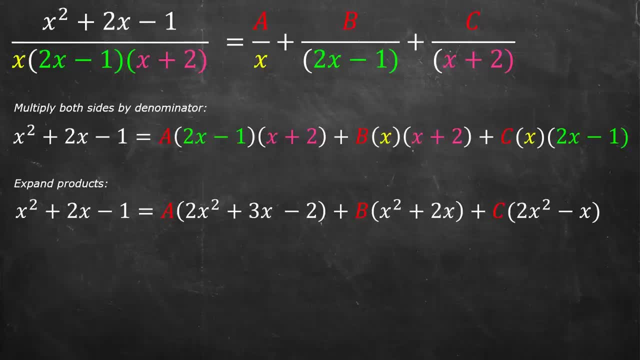 But I want to now focus on the x squared, the quadratic terms, the x terms, the so-called linear ones, and the constant terms. That is, I'm just going to rearrange the right-hand side, but I'm going to rearrange it in terms of powers of x. So there's x squared and 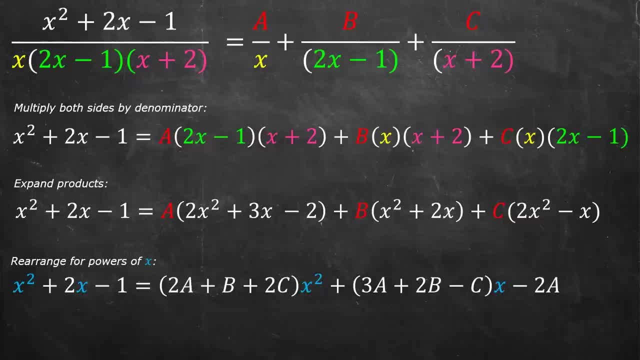 then all the things that multiply by the x squared. It looks like a- 2a and a b and a- 2c. Then I'm going to add all the things that multiply out by the x term, the linear term, and then finally I leave whatever constant remains. It looks like a- 2a and a- b, and. 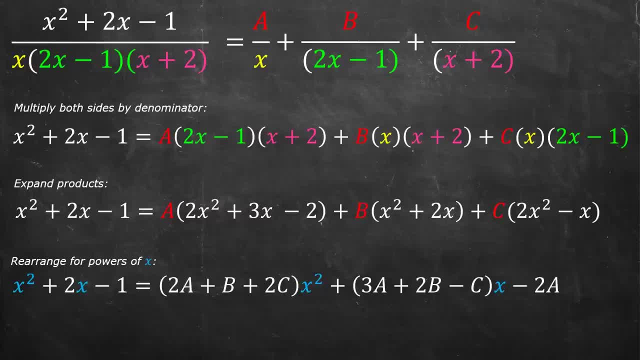 a 2a, It looks like a- 2a and a b and a 2a. So this isn't any calculus, It's just algebra, It's just reordering, It's expanding everything out, seeing what the values are multiplied by x, squared x and constants respectively. 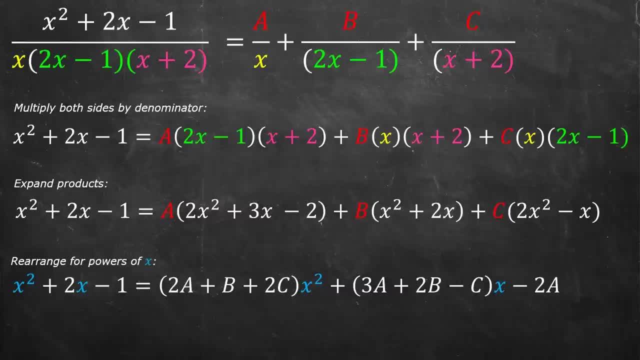 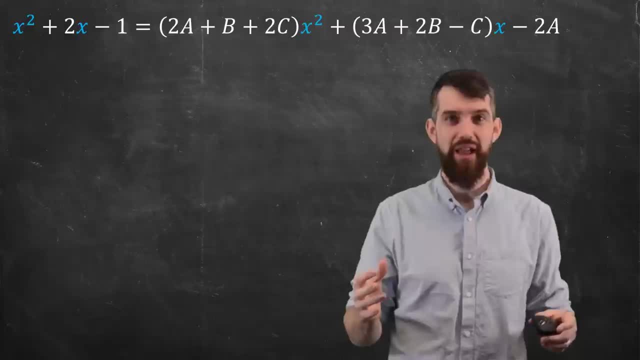 and then factoring them in terms of the x, squared in terms of the x and in terms of the constant term. All right, so let me keep my focus on that. All right, once again, there's space for me. Now, if I look at this equation, I see one. 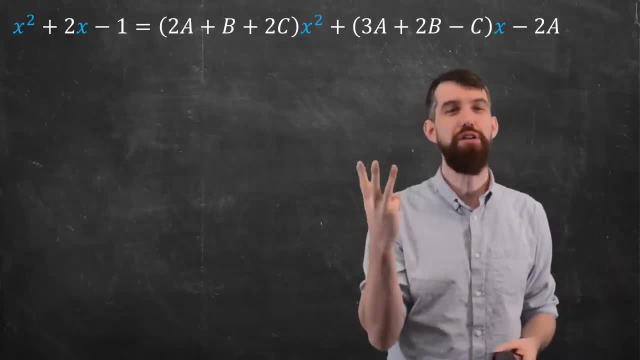 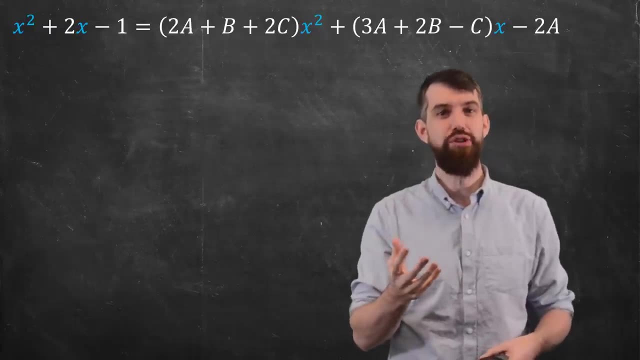 equation on its face, but in truth there's three different equations here, And the idea is that this quadratic, the x squared terms, the linear, the x terms and the constant terms. they sort of vary independently, Like, for example, if I plugged in x equal to 0 here, all that would remain is the constant. 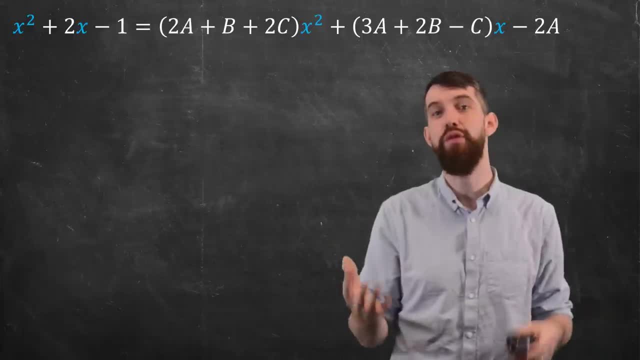 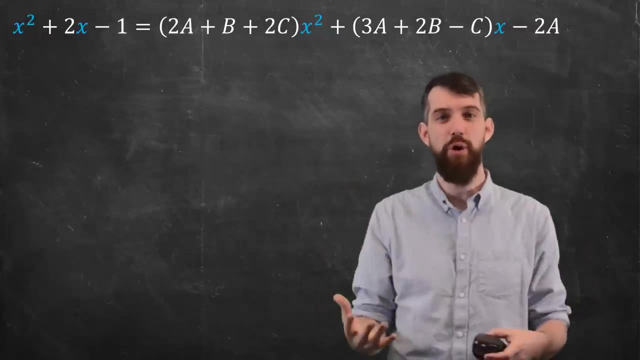 terms. So that would mean that the constant terms all had to be equal. There was an equation for those. And then, as I varied the x or I varied the x squared, the coefficients of the x would have to line up. the coefficients of the x squared would have to line up, So I can split. 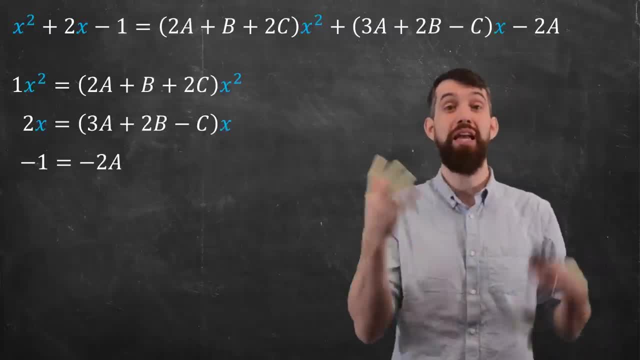 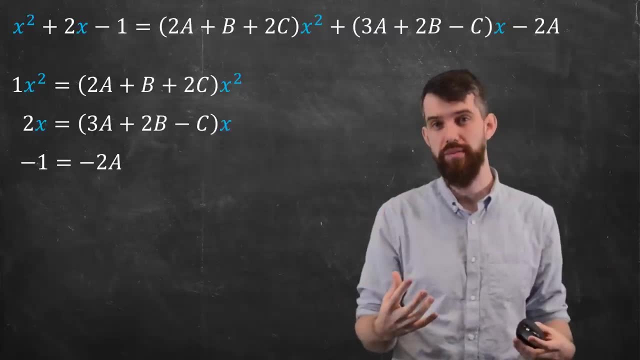 this into these three different equations: One equation which is relating the coefficients of x squared, One equation that's relating the coefficients of x And one equation that's relating the constant terms. And then, in fact, I can actually just get rid of the x and the x squared here to have 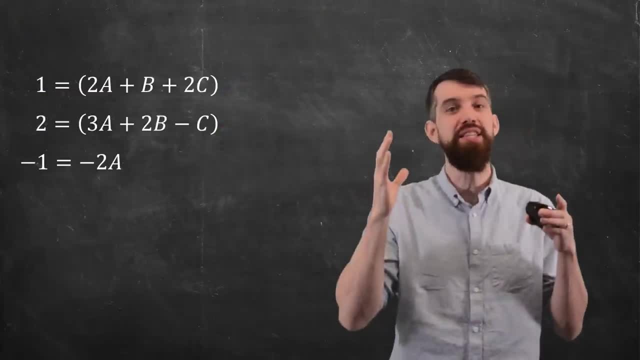 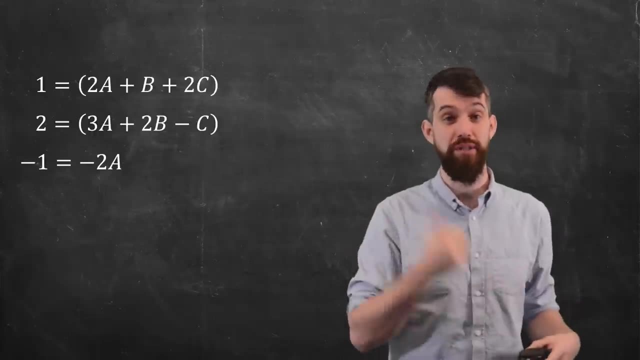 three different equations And, if I get rid of the original, this is the system of equations I want to solve. There are three equations and there are three unknown variables: the a, the b and the c. Now how do you solve systems of equations like this? 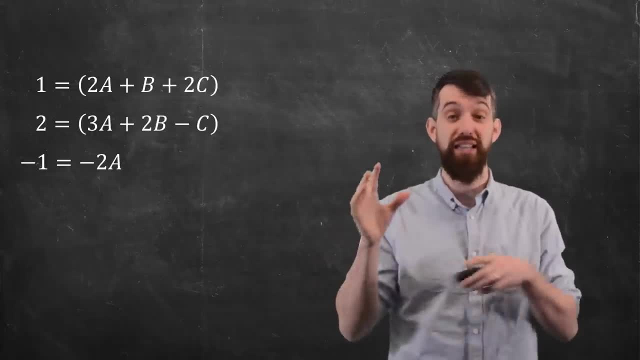 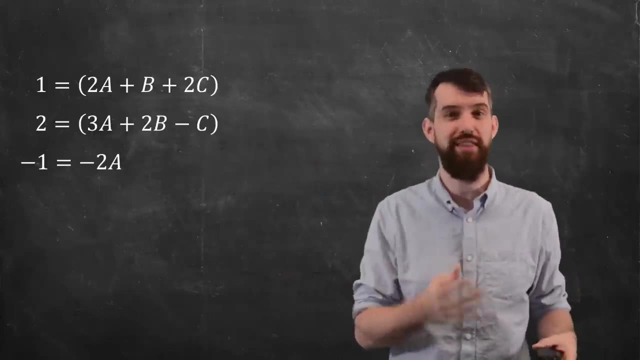 Actually, I'm going to teach a course, I believe in the summer- an online linear algebra course, and one of the things it will do is show a systematic way where you can solve systems of linear equations like this. Always plug it. You should register for it in the summer. 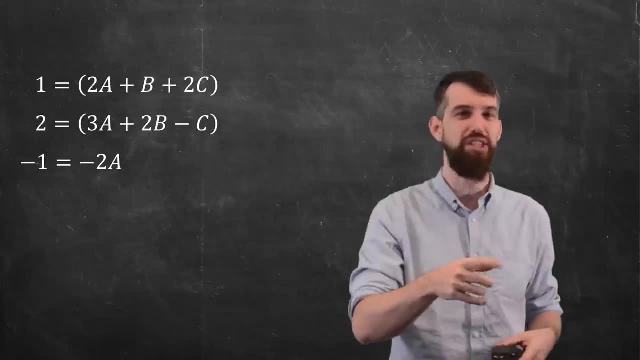 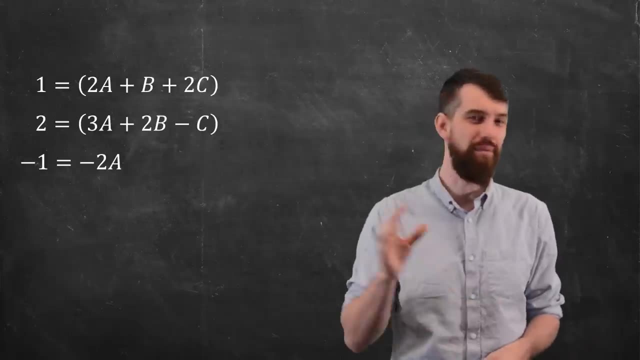 However, for our purpose, I would just encourage you to pause and just sort of ad hoc try to solve it. See whether you can get the a, b and c from this linear system of equations Here. I'll do it relatively quickly for you. 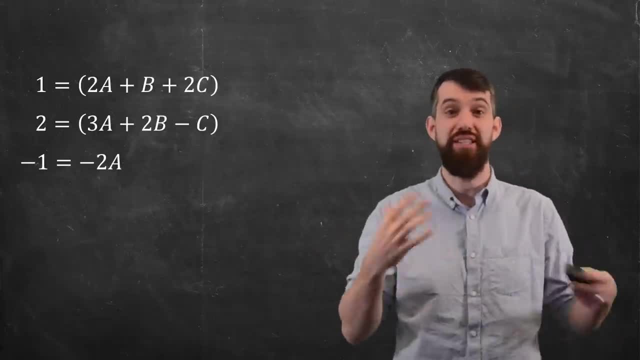 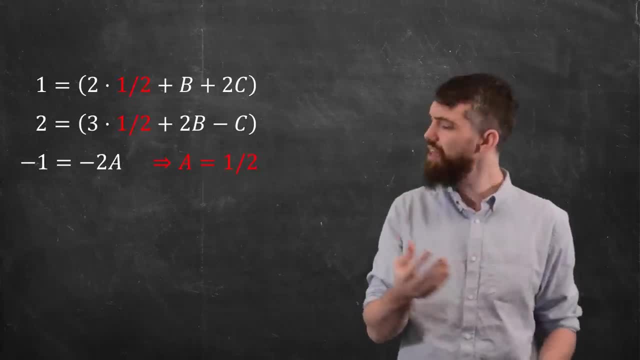 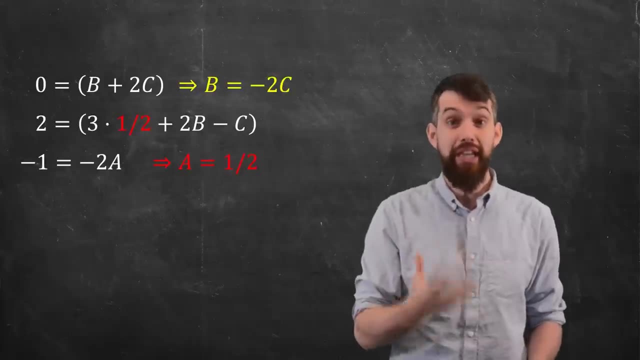 So I can move one half into the spots where there was going to be the a and the two different equations. If I then look at the top equation, OK, I'm going to put the constants back together. So zero is equal to b plus two c, and this is going to give me a relationship that b. 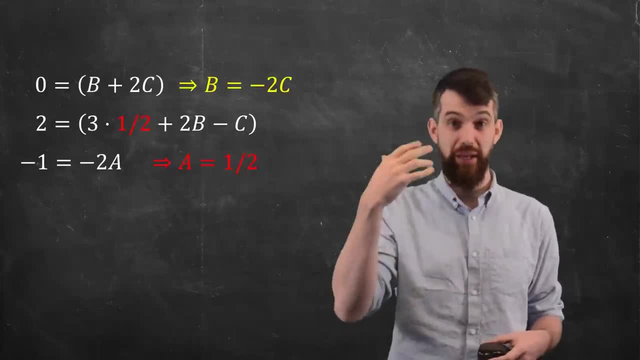 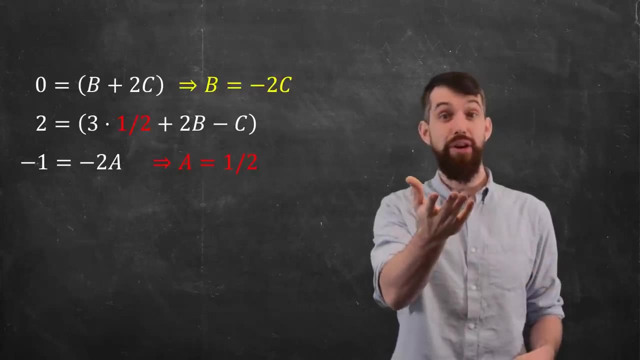 is minus two times c. All right, So that was manipulating the top equation. If I now focus in on the second equation, here I have a, b and a c, But from the top equation I have this relationship Where there's a- b. here I can plug in minus two c. 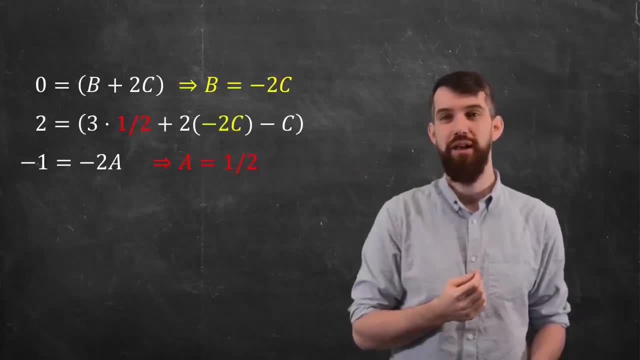 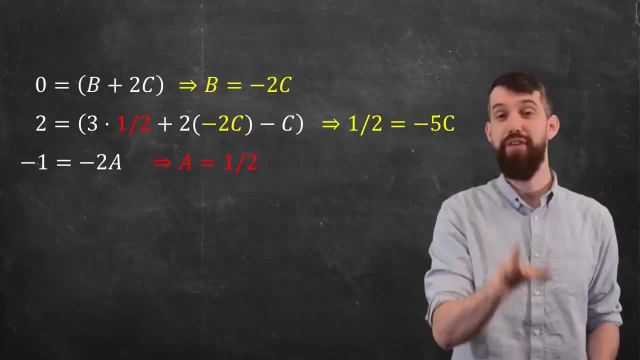 So let me do that. I'll replace my a, I'll replace my a, I'll replace my a, my b with the minus 2c. And now the second equation is all in terms of c values. So if I collect the c's and collect the coefficients, I get 1 half is minus 5c. And if I go and divide out, 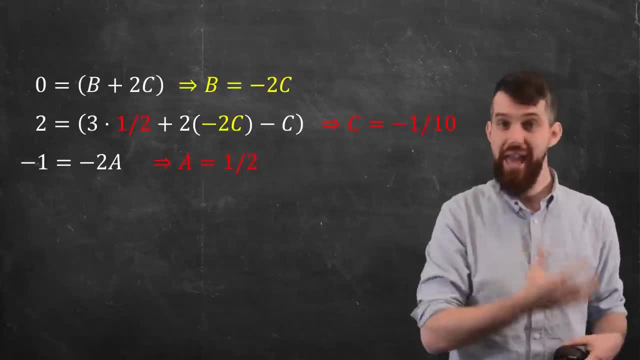 I get. my c is minus 1 tenth. So now I know my a, I know my c If I look at the top equation again- remember I had that relationship- b is minus twice c. So if c is minus 1 tenth then my b is going. 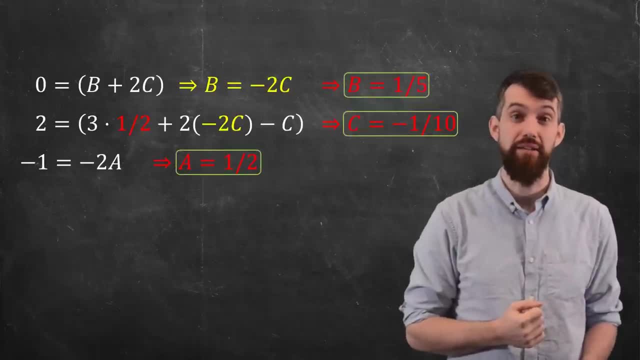 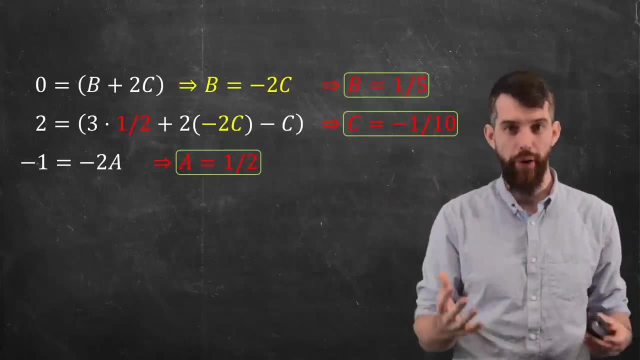 to be equal to 1. fifth, And now I have my a, b, c's, So that was my particular sort of ad hoc way of solving this system of linear equations. It's just a bunch of algebra, All right. where are we? 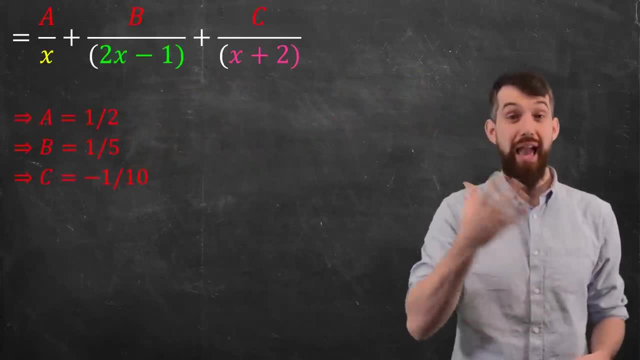 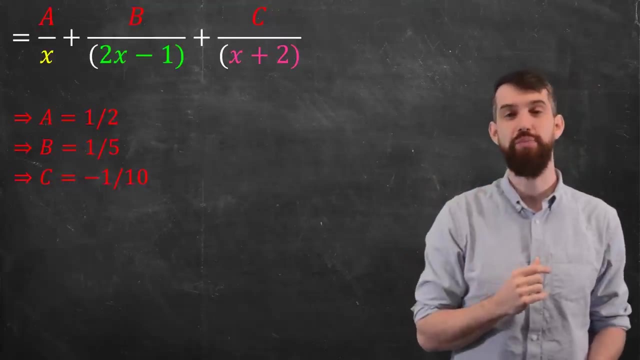 We solved the a b c's And I'll remind you that the a b c's were the a b c's in this form: a over x, b over 2x minus 1, and c over x plus 2.. I was trying to figure out what the a b c's are. 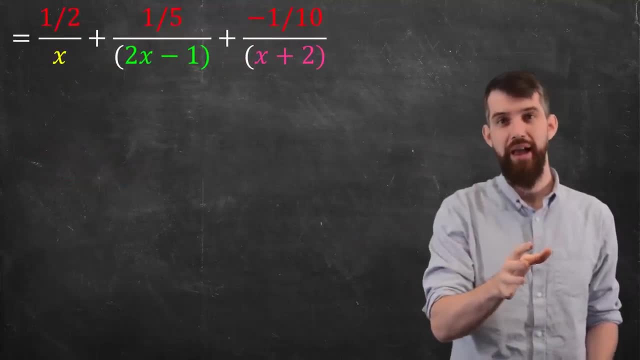 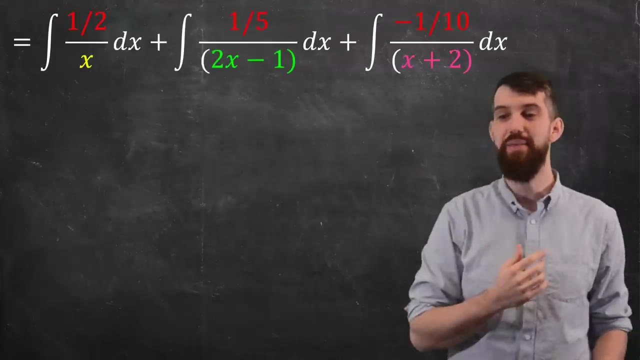 I now know what they are, so I can go and plug them in And, finally, I am trying to integrate something. So what do I want to do? I want to go and replace this with something that I am integrating. I am integrating this with something that I am integrating, And I am integrating this. 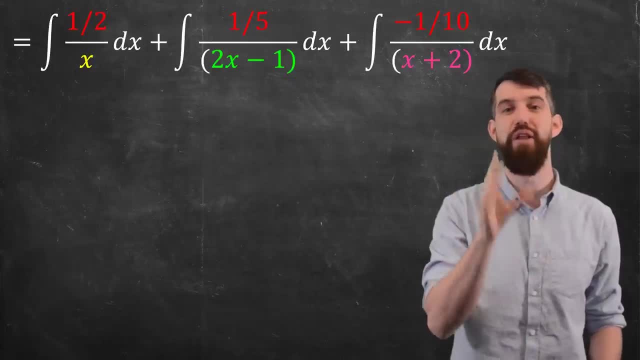 with something that I am integrating, And I am integrating this with something that I am integrating, And I am integrating the 1 half over x, I am integrating the 1 fifth over 2x minus 1, and so on, Each of. 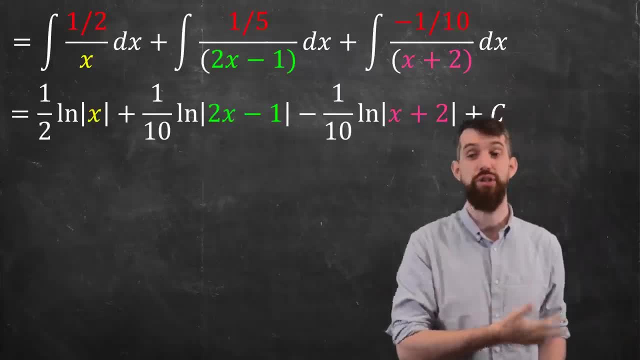 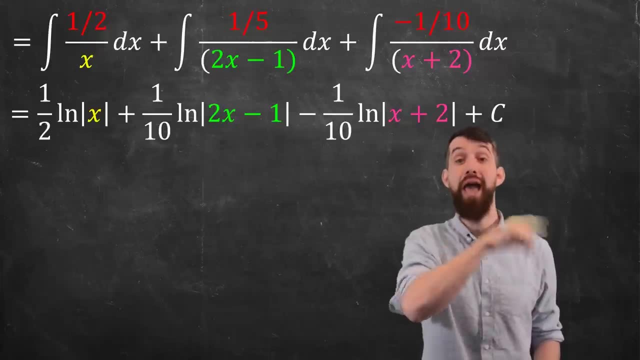 these is going to be a logarithm, a logarithm with a different u substitution. So what do I get? 1 half, logarithm of x. Then I get 1 tenth, the 1 fifth, And then there's another 1 half that comes. 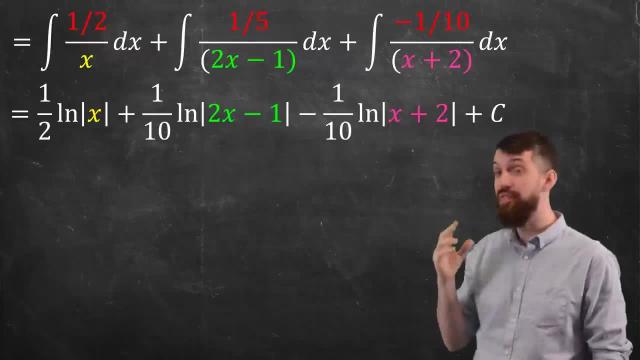 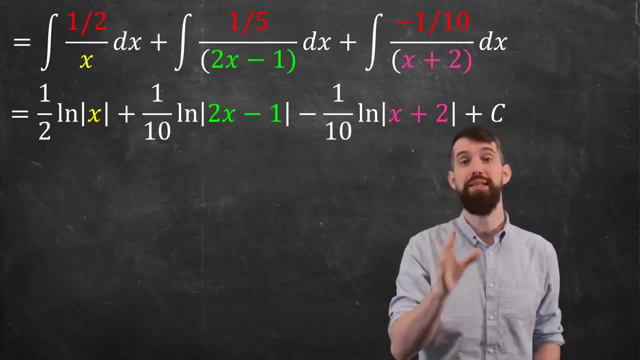 when I do my u substitution with u equal 2x minus 1.. So 1 tenth, this logarithm of 2x minus 1 in absolute values, And then, minus the 1 tenth, the logarithm of x plus 2, all plus c. So 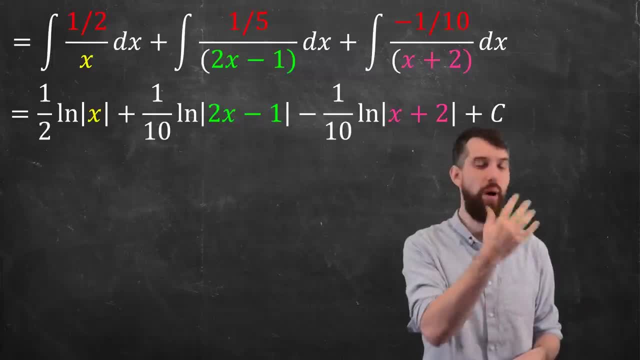 indeed I have gone from that original rational function, the polynomial over polynomial. I split it up using this partial fractions algebra. I figured out my coefficients by a, b, c, And when I did that I got something I could integrate. And now I've gotten the function after I integrate. 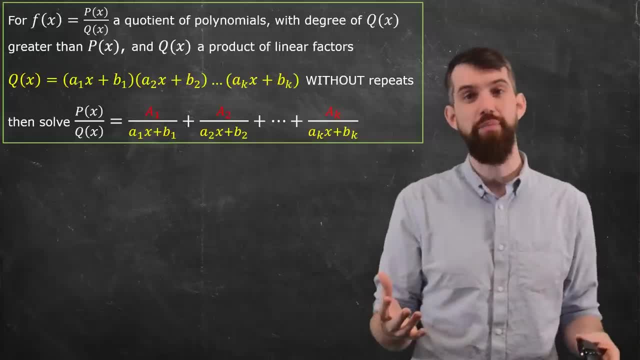 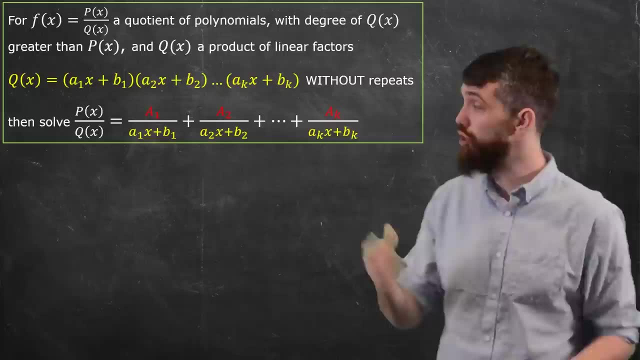 Now the method that we've talked about. it does work generally, but there's a couple different cases, And we've only seen one of them in this video, That is, if I'm looking at a so-called rational function, a quotient of polynomials, a p of x over a q of x. 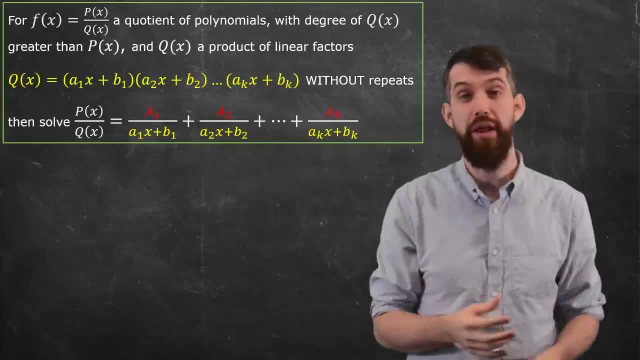 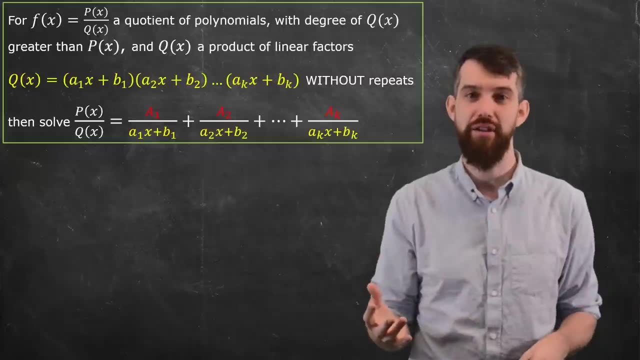 I'm asking: is that q of x the denominator? can I write that as a multiplication of a bunch of non-repeating linear factors? That's what we had before We saw it was like an x and then a 2x.